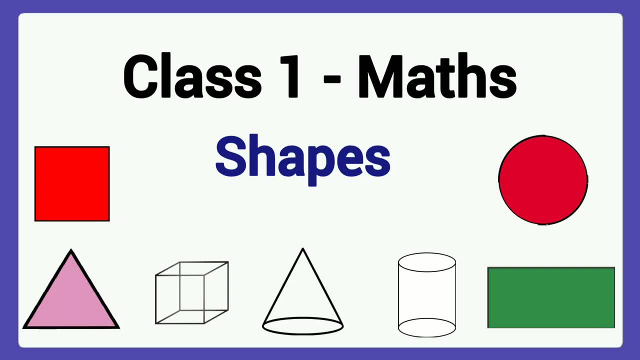 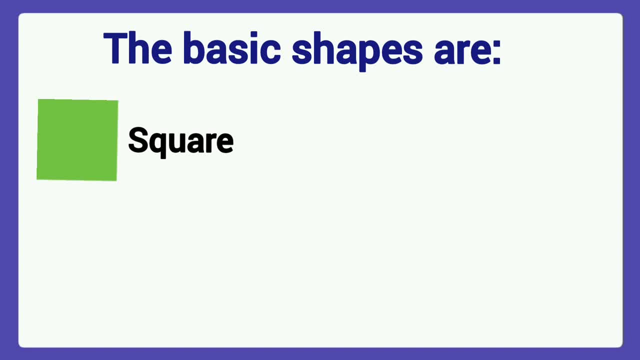 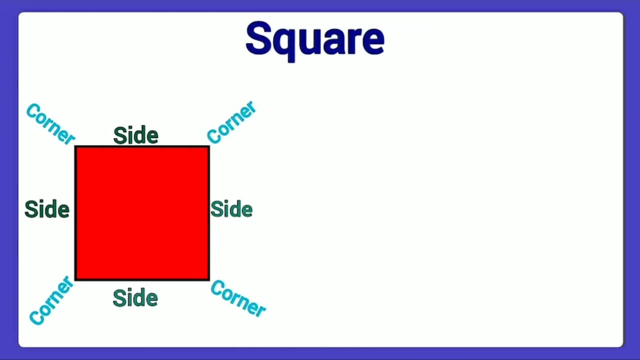 Today we learn about shapes. There are four basic shapes: Square, rectangle, triangle and circle. These are plain shapes. Here first we learn about square. Look at this picture. How many sides are here? One, two, three, four? Then count how many corners are here: One, two, three, four. That is square shape has four corners and four sides. And check these four sides: Yes, it's, all sides are equal. 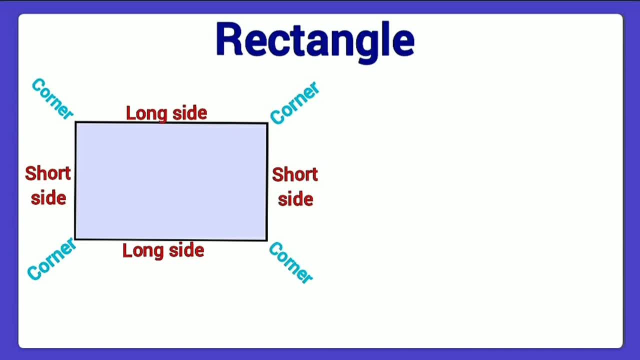 Next, one rectangle. Count the sides One, two, three, four And how many corners. One, two, three, four. That is rectangle has four corners and four sides. And look at this picture: It has two long sides and two long sides. 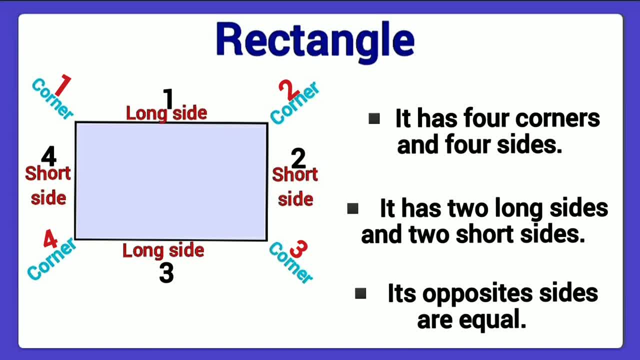 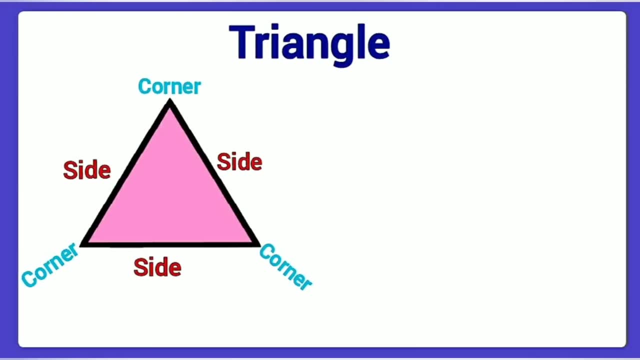 It has two short sides. Next, its opposite sides are same length, Or we can say that its opposite sides are equal. Next, one triangle. Look at this picture and count how many sides are there- One, two, three, Three sides- And how many corners. 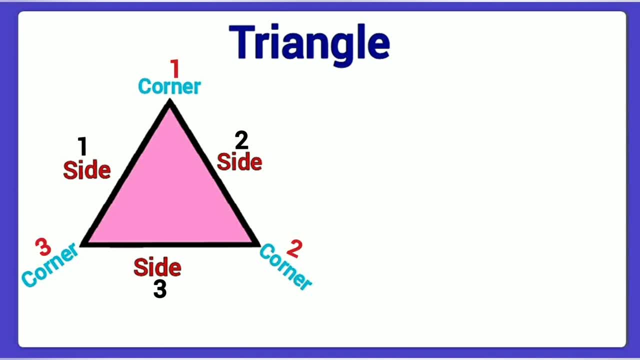 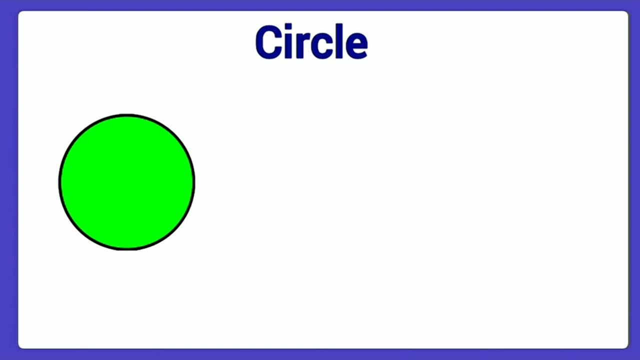 One, two, three corners. So the triangle has three corners and three sides. Next circle: Look at this picture. Is there any sides or any corners? No, it is a curved shape, So it has no corners and it has no sides. That is, it is round shape figure. It has no corners.